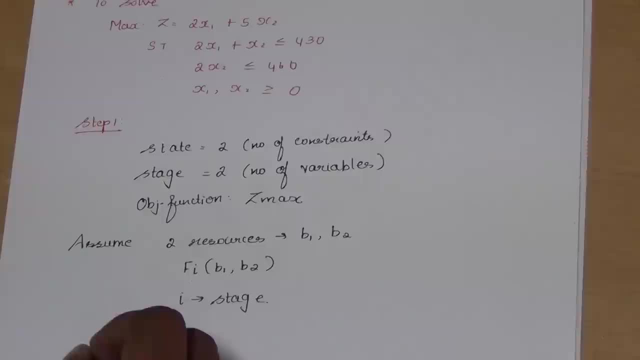 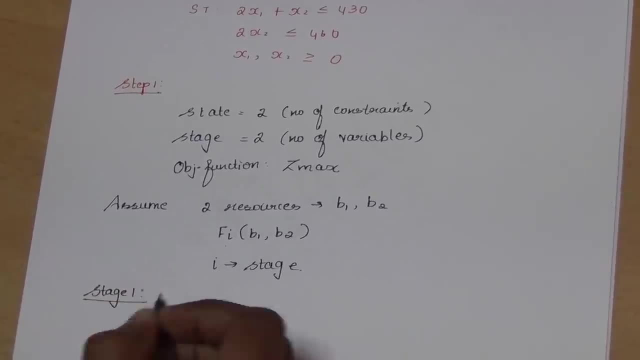 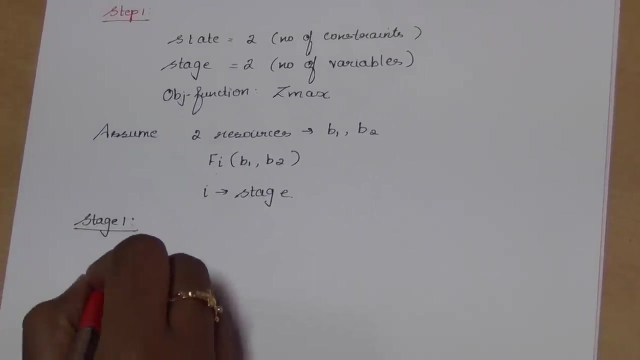 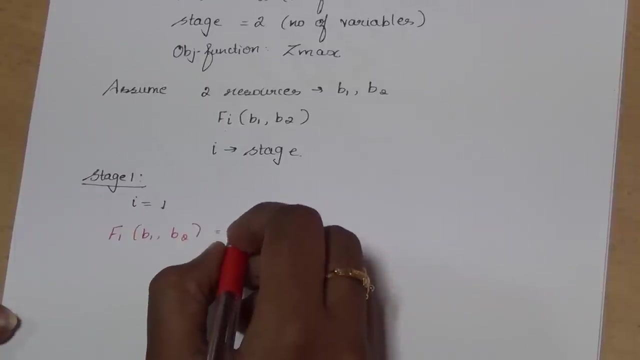 stage. Now we have two stages, so let's see two stages separately. Stage 1. So therefore, i is equals to 1.. So let's frame the function f1 of b1 comma. b2 is equals to from the objective function. we will be framing the function, So it is maximum of, since it is the first stage. 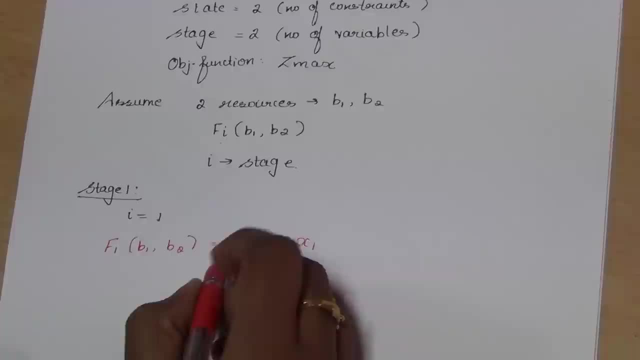 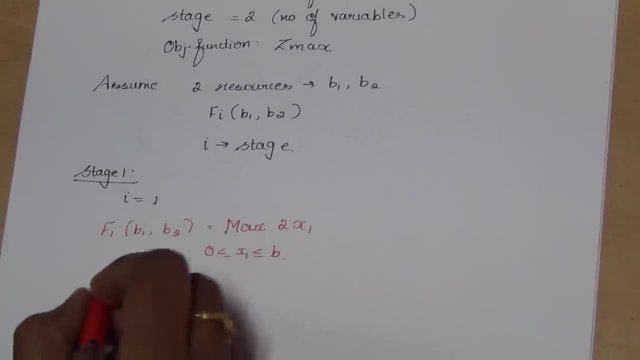 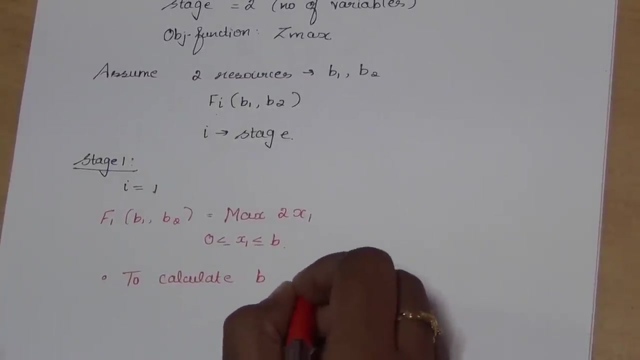 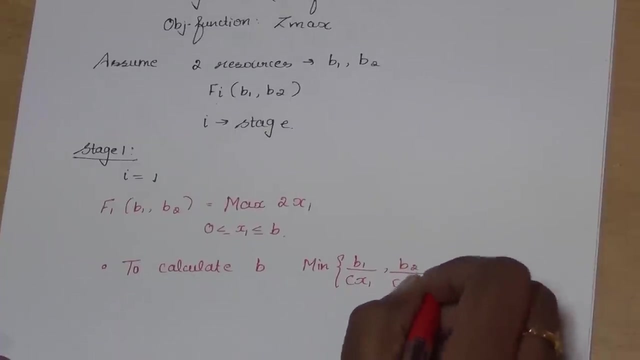 we will use only the first variable, 2x1, whose limits varies between 0, less than or equal to x1, less than or equal to b. So in this first step we have to calculate the value of b. To calculate b, the formula used is minimum of b1 comma, cx1 comma, b2 comma- cx2, where b1 and b2 are the resources. 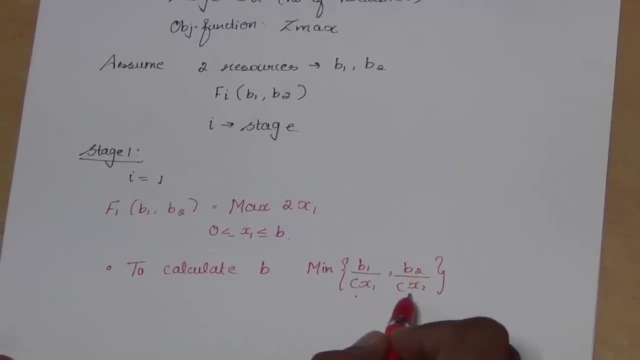 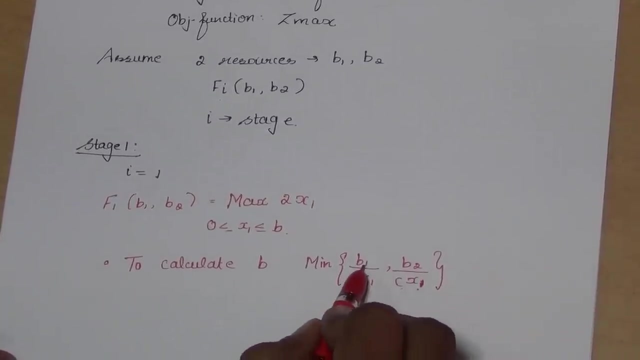 and cx1 is the coefficient of x1.. So we have to calculate the value of b. So we have to calculate the value of b and cx. sorry, this is also x1 and cx1. this is the coefficient of x1 of the second constraint. b1 will be the right hand side of the constraint number 1.. So which? 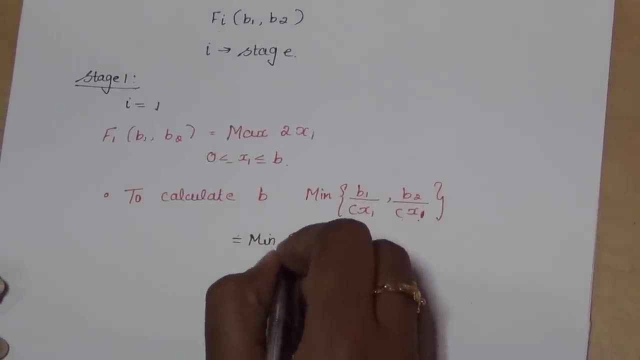 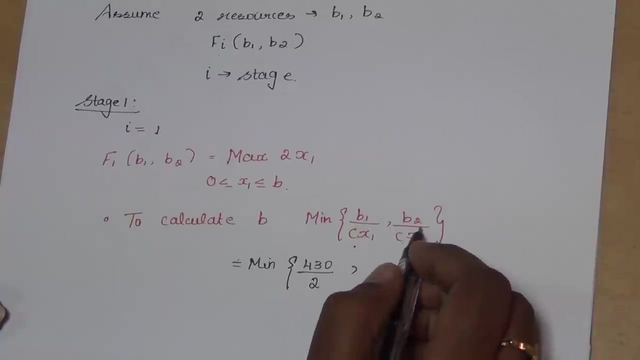 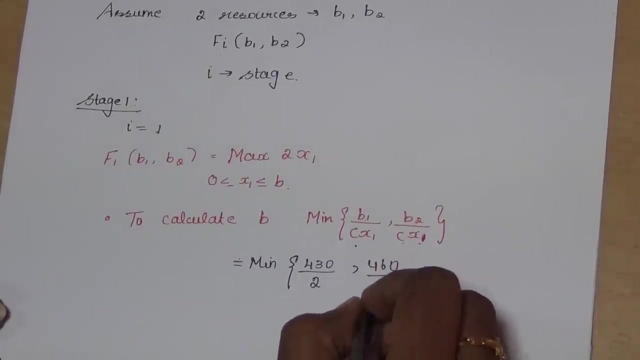 will be: minimum of right hand side of the constraint number 1 is 430 by the coefficient of x1 of the first constraint, which will be 2 comma b2, right hand side of the constraint number 2: 460.. Since there is no x1 in the second constraint, it will be 0.. As we solve. 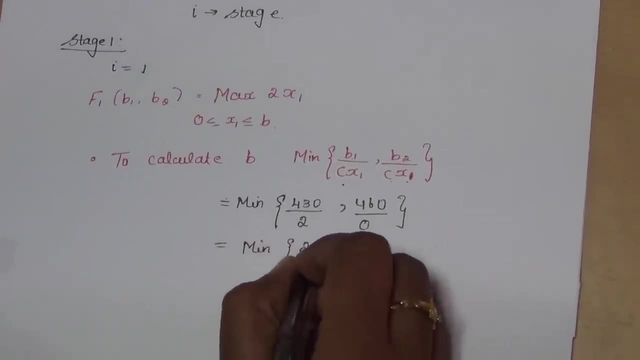 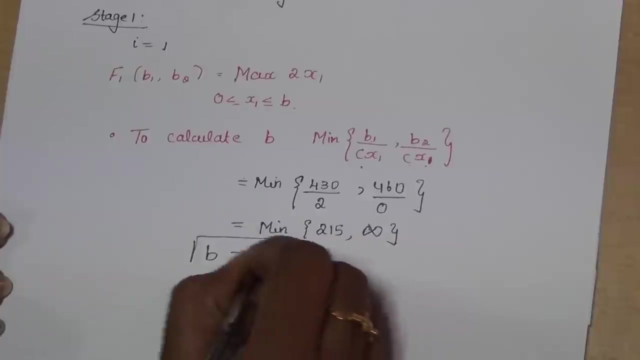 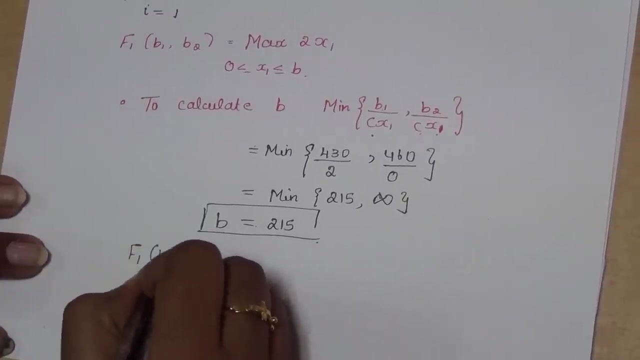 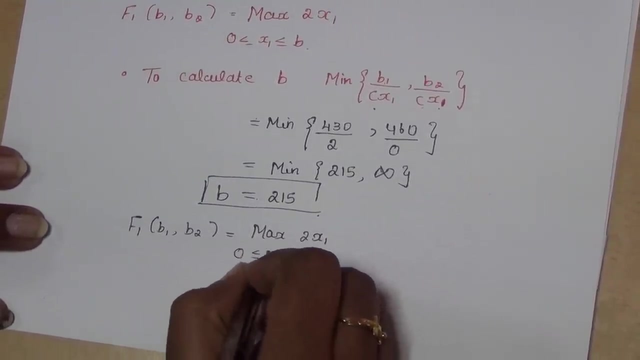 this, it results in minimum of 215.. Anything divided by 0 will result in infinity, So the final value is 215.. We substitute this b in the function f1 of b1, comma. b2 is equals to max of 2x1, where limits varies between 0x1 to 215.. Now we have to find the value. 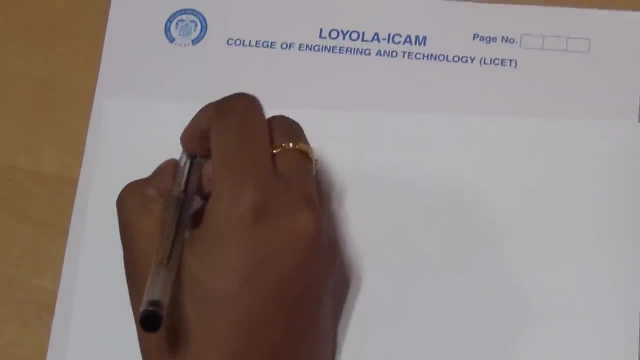 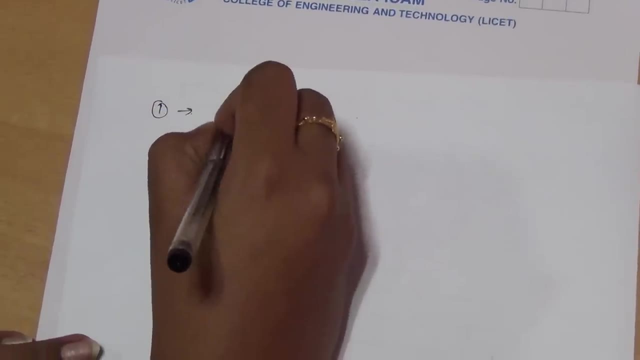 of x1.. So to find the value of x1 we have to find it from the constraint First. from the first constraint the value of x1 results in: x1 is equals to 430 minus x2 by 2.. Since we do not, 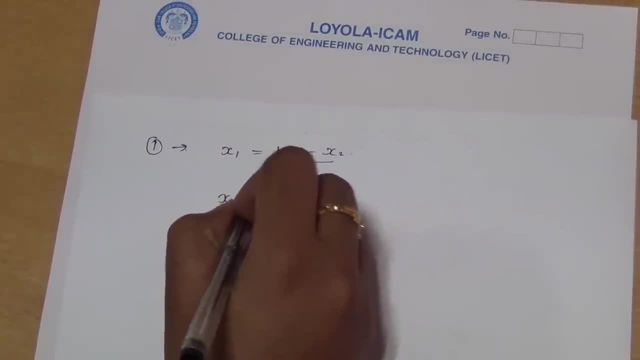 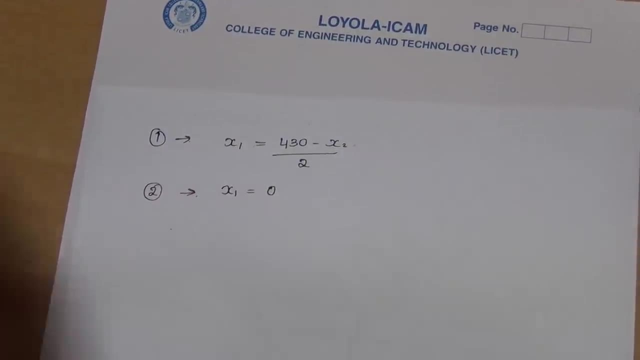 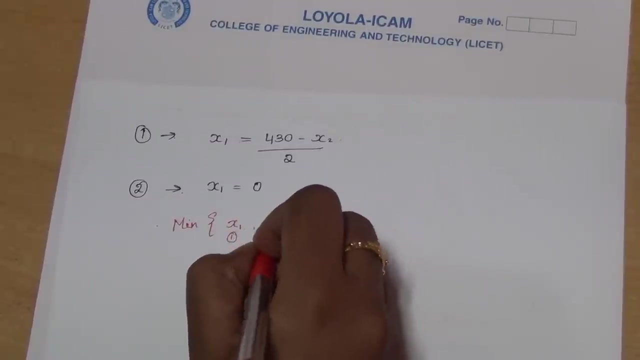 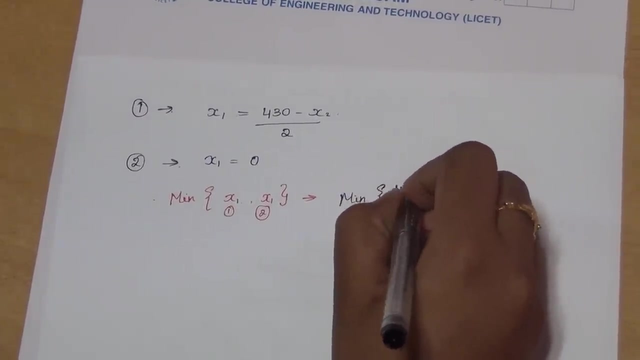 have the x1 in the second constraint. from the second constraint the value of x1 will be 0. So to find which x1 value to be used, the formula used is minimum of x1 from the constraint number 1. And minimum of x1 from the constraint number 2.. So minimum of 430 minus x2 by 2 comma 0.. 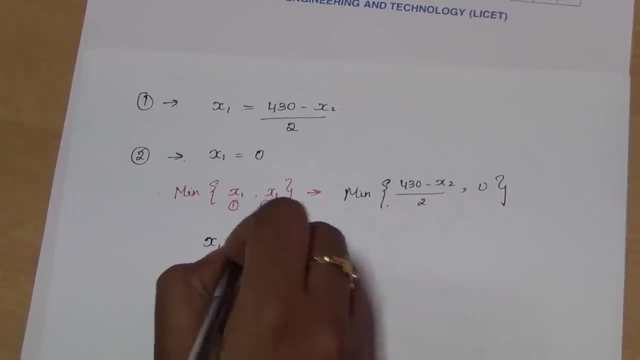 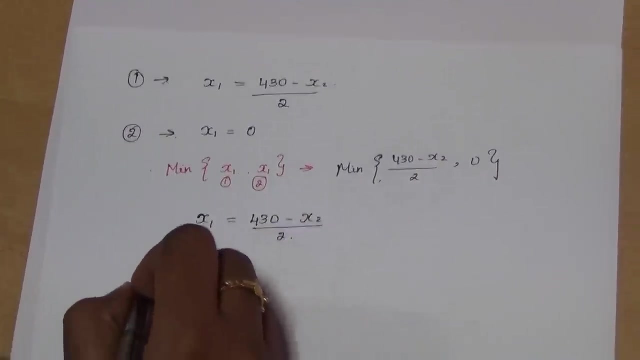 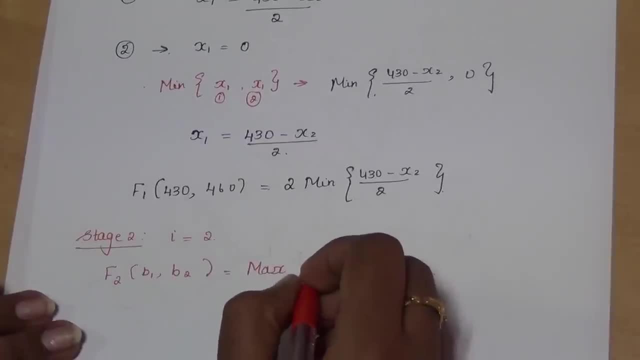 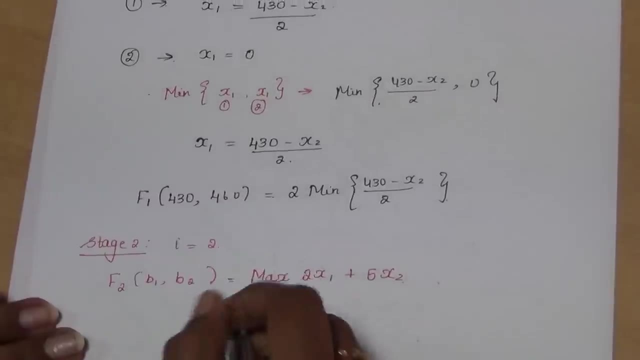 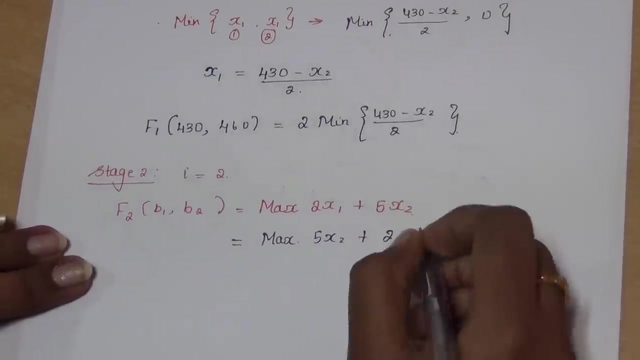 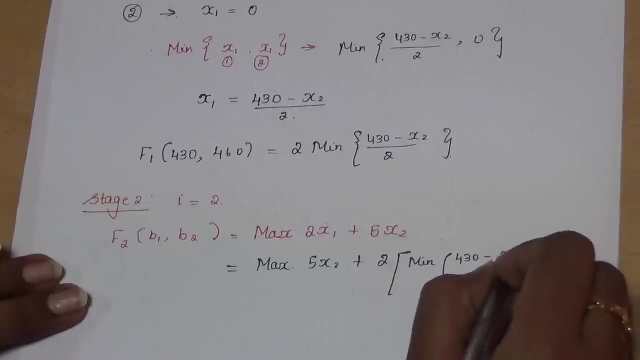 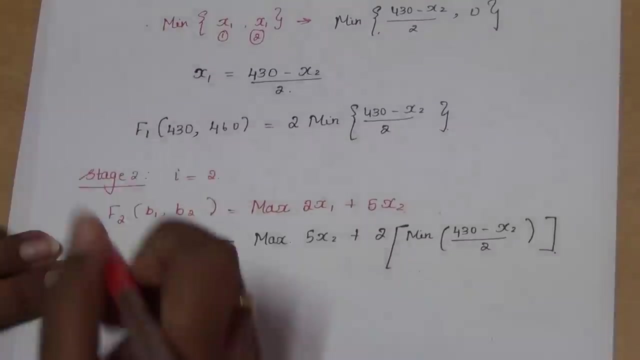 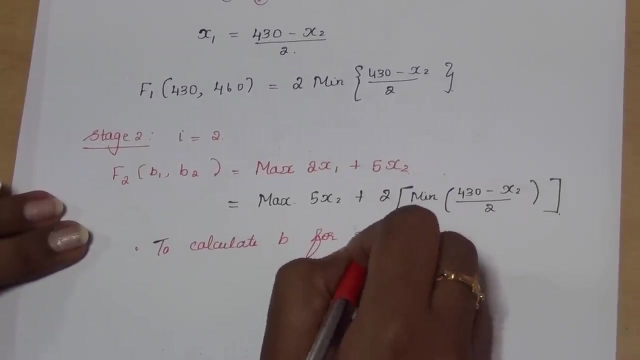 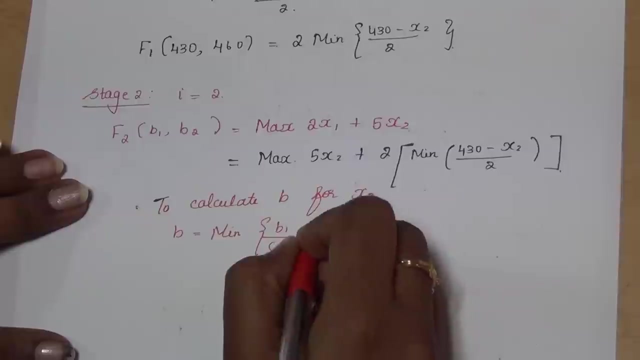 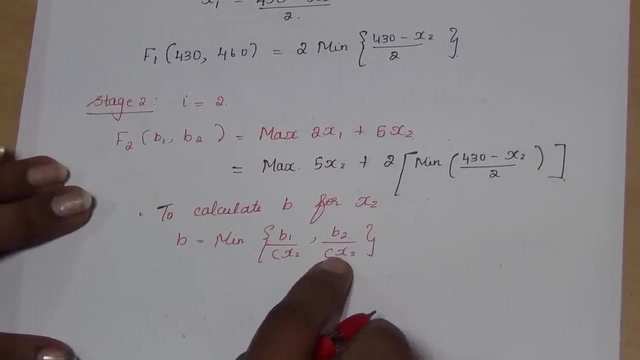 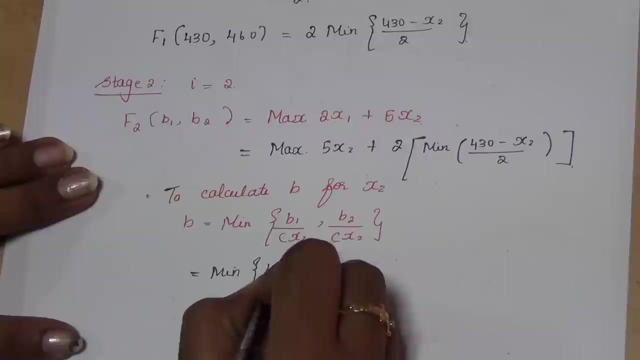 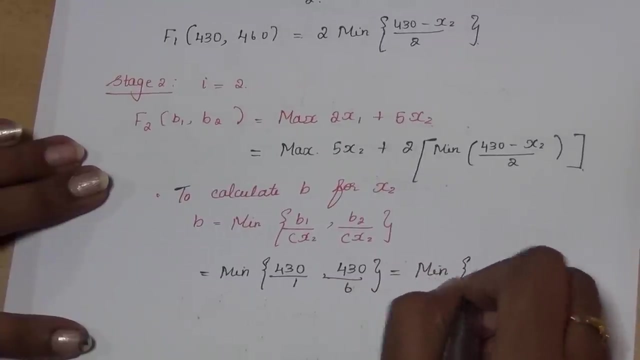 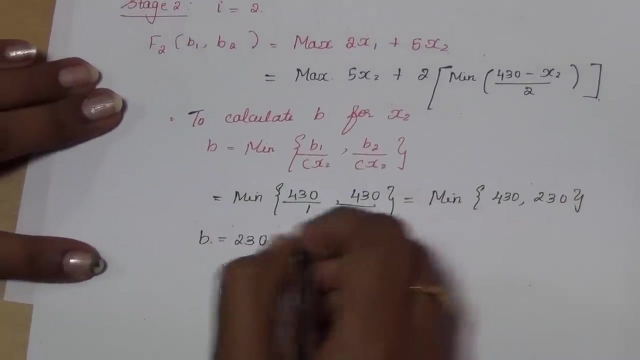 1, 430, 6.. By solving this you will get minimum of 430, 230.. So the final answer is: B is equals to 230.. Sorry, this will be 460.. Now let's substitute in the function we have known. 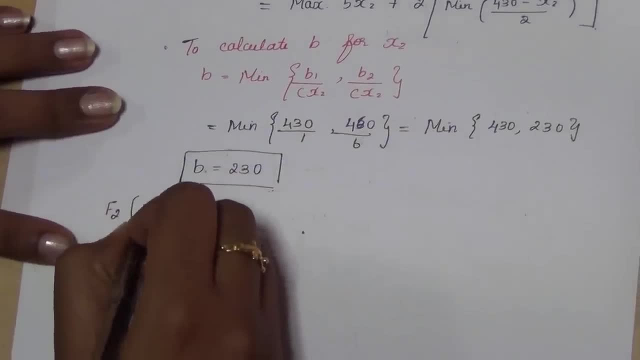 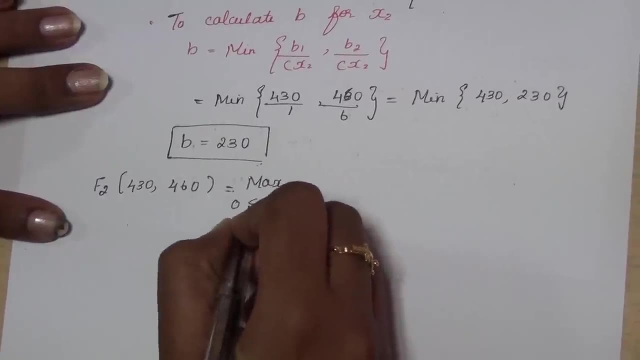 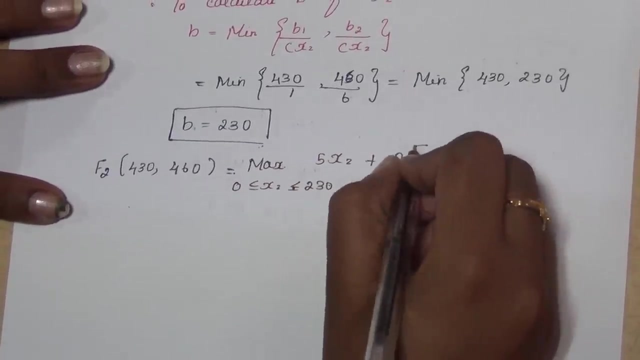 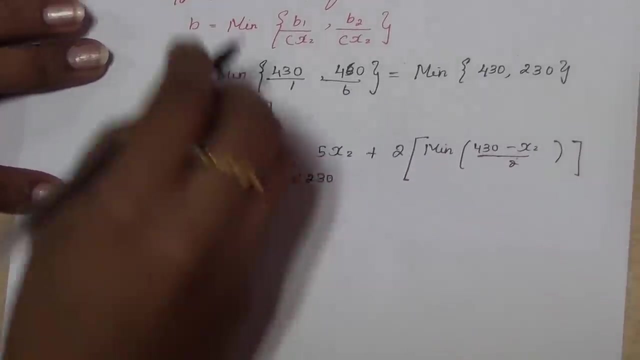 it F2 of so B1 value will be 430,. 460 is equals to maximum. the limit varies between 0, X2 less than or equal to 230, 5X2 plus 2 into minimum of 430 minus X2 by 2.. So to: